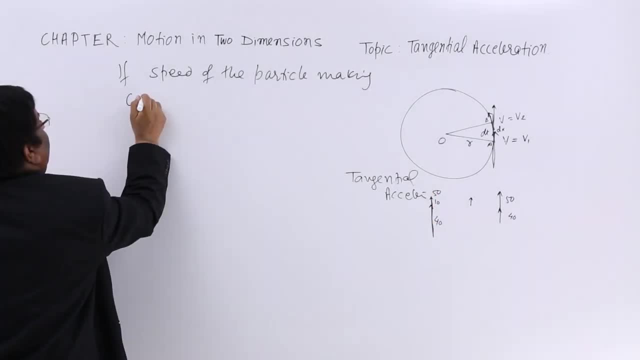 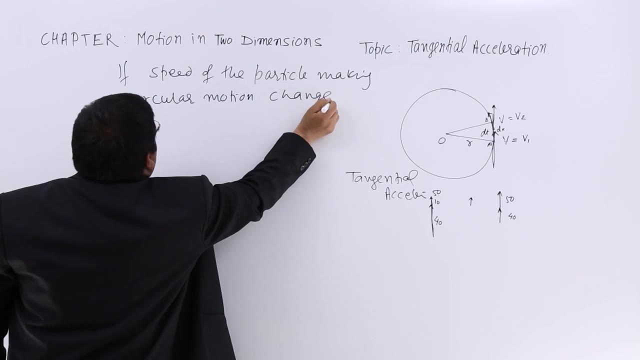 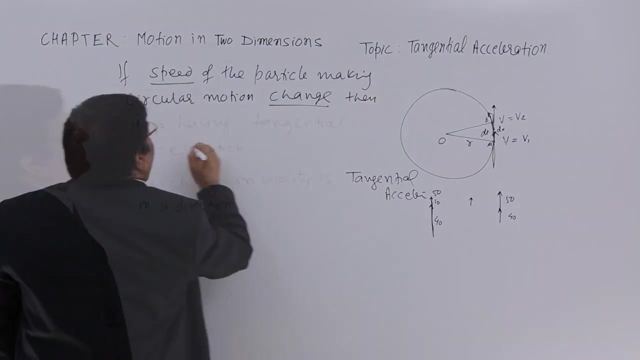 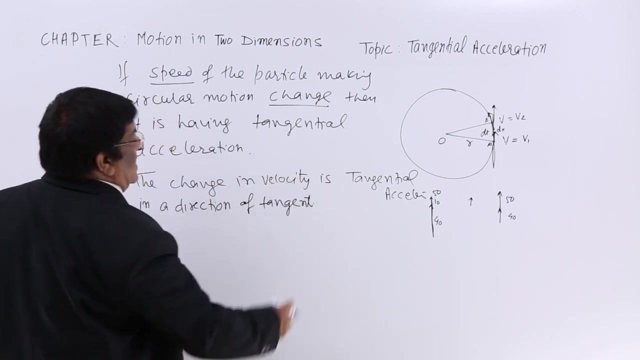 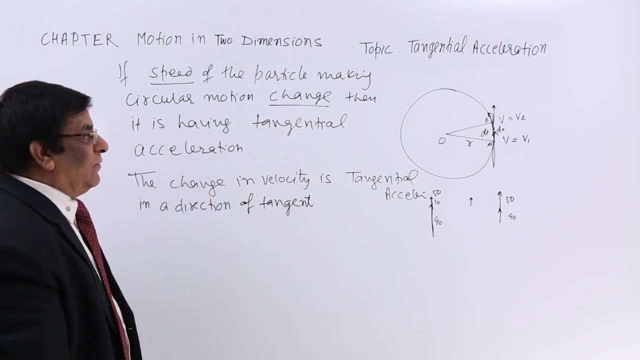 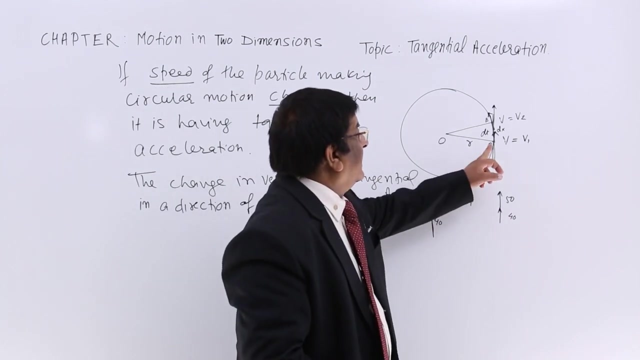 as tangential acceleration. If speed of the particle making circular motion change, what change? Speed change, then it is having tangential acceleration. b: change in velocity is in direction of tangent. So this is tangential acceleration. What is its direction along the tangent? Now, if this particle, which is going at a speed of 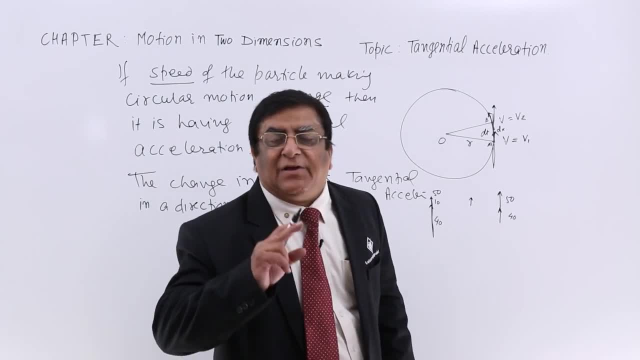 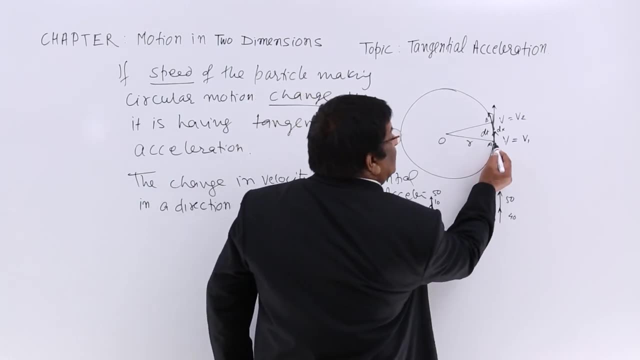 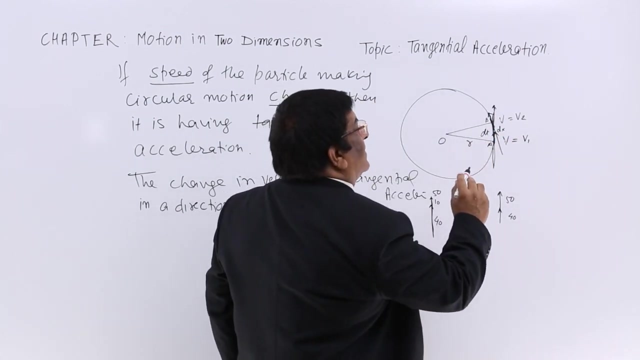 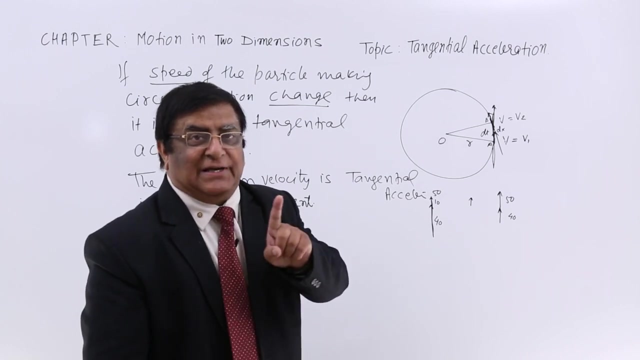 40 here and 50 here. is it having centripetal acceleration or it is not having centripetal acceleration? Answer is: because it is changing its direction. Because it is changing its direction, therefore, it has centripetal acceleration, Because it is changing its direction from. 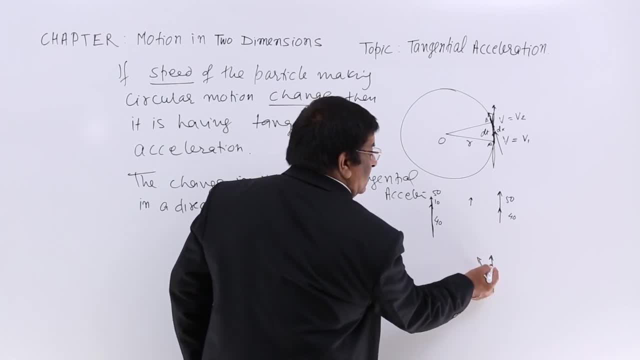 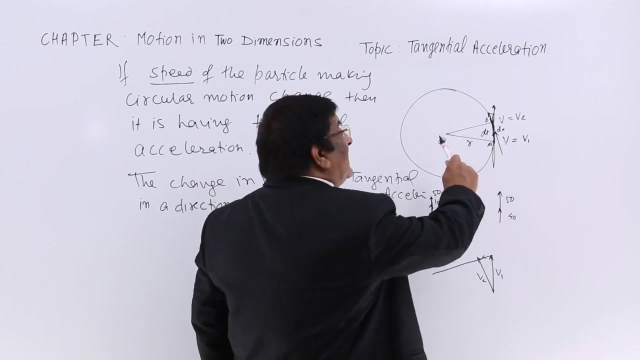 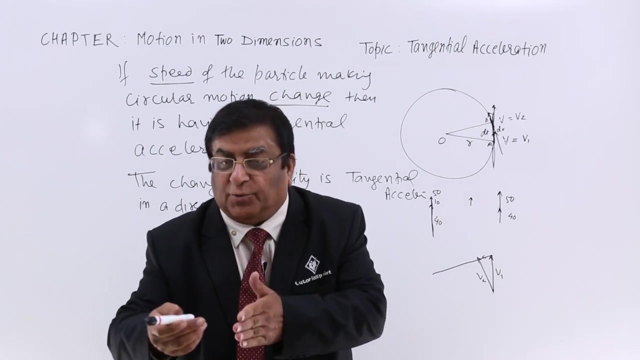 V1 to V2.. This may be a little less or more, does not matter. This is the change and this change is always normal. Now, if there is a change in the speed also, then we say there is acceleration in the direction of motion of the motorcycle, Because this 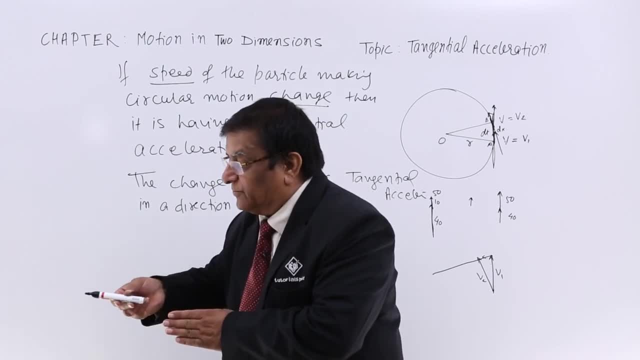 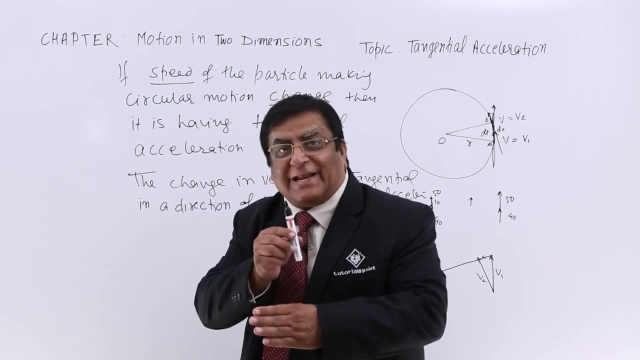 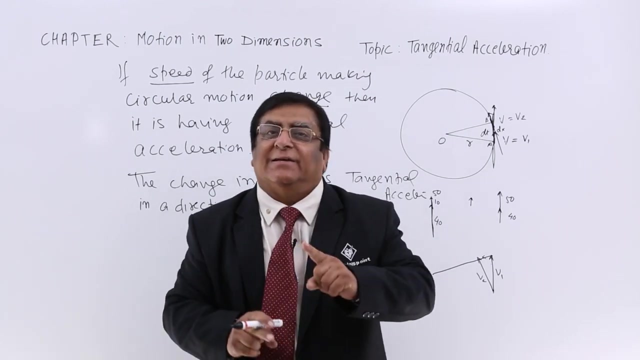 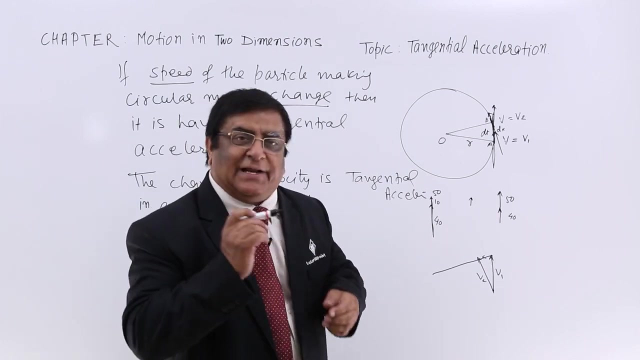 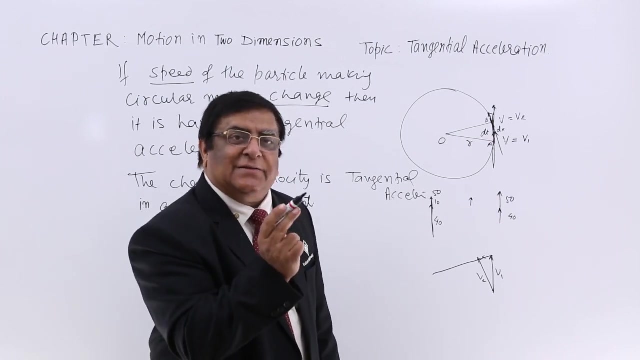 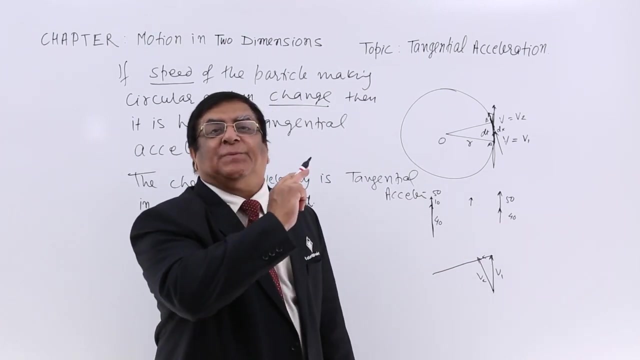 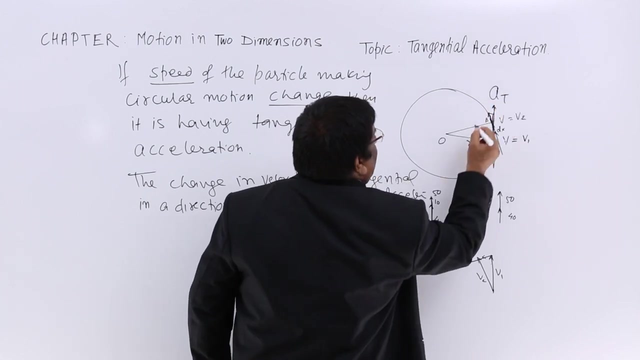 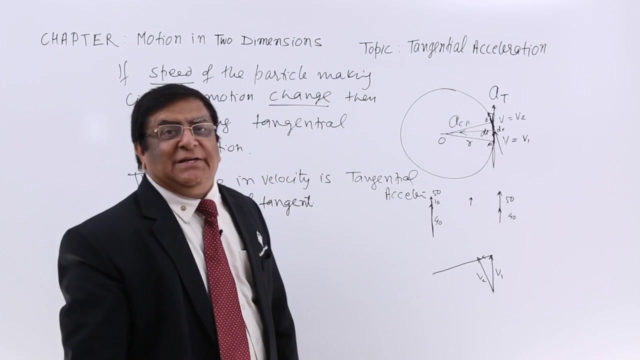 motion was 40,, 41,, 42,, 43,, 44.. In the direction of the motion the velocity is increasing, so it has one acceleration in its direction. This is acceleration tangential and this is acceleration centripetal. So a particle. 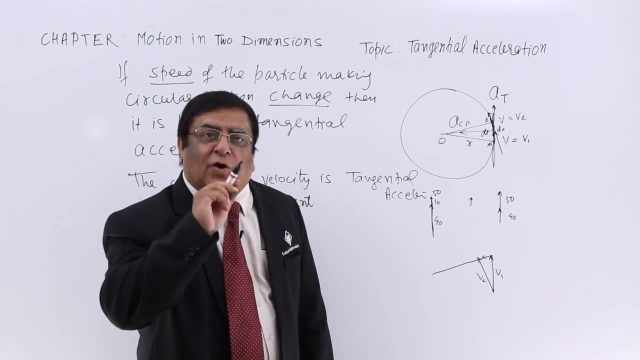 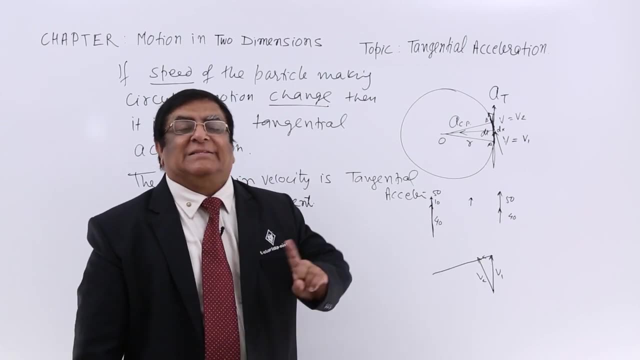 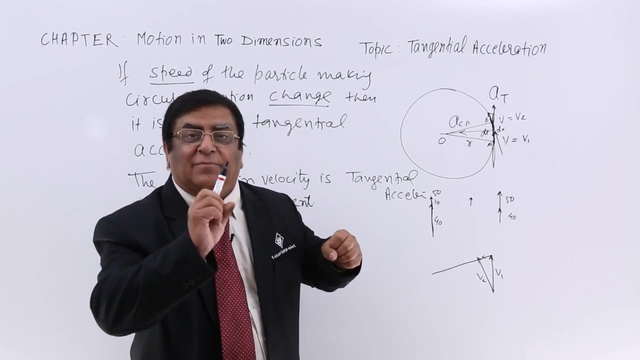 which is making a circular motion because it is turning at every point. it is supposed to have centripetal acceleration. At the same time, if there is a change in its linear speed, then we can say it is applying brake, it is accelerating. At that time there is a change.